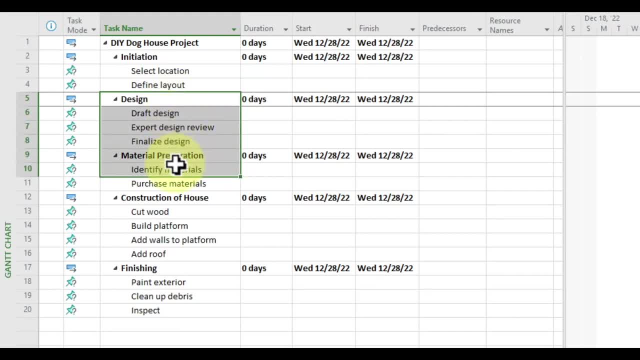 The second and the third phases are drafting the design and identifying and purchasing our materials. The fourth and the fifth phases are constructing and finishing out the house. Now it looks like we're missing a few key tasks for testing the floors, the wall stability and roof leaking before we can actually mark the house as fully completed. 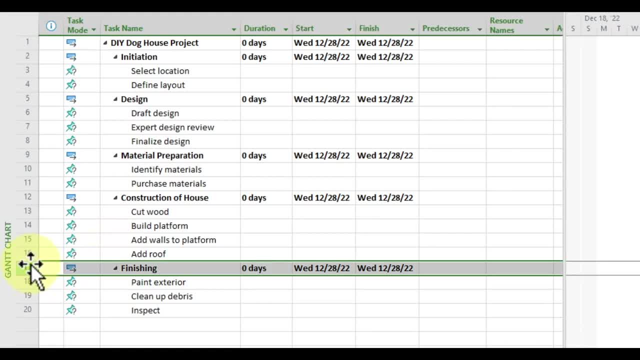 So let's insert a group of tasks after add roof. To do that, hover your mouse to the leftmost column with the numbers and drag it down to select add roof, Right click and select insert task. We want this first task to be the section header. 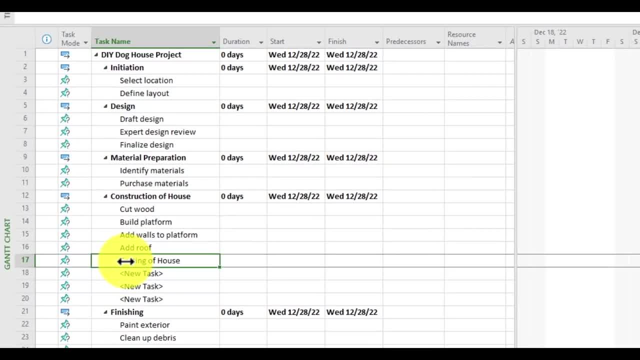 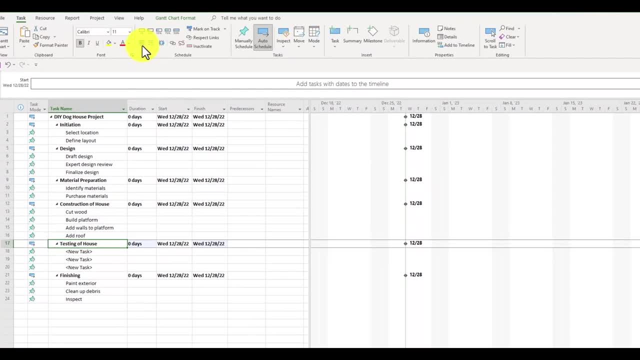 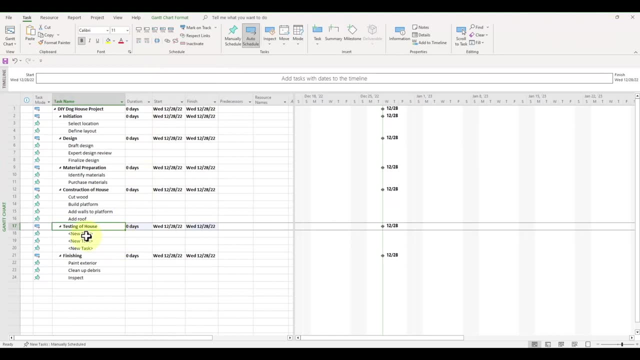 Let's call it testing of house And let's outdent it by pressing alt plus shift plus left arrow. If you ever need to indent or outdent a task, use these buttons here, which are a part of the schedule group underneath the task tab. Now, as part of testing the house, we want to complete 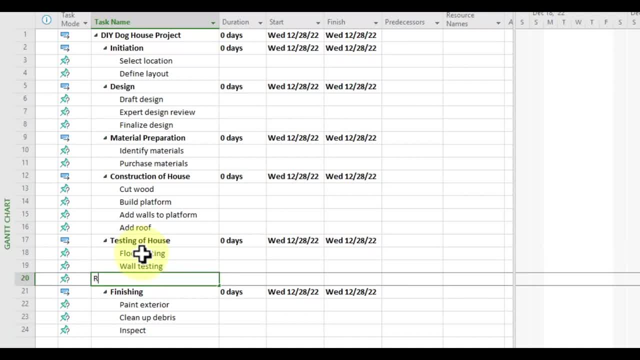 floor testing, Wall stability testing and roof waterproof testing. It looks like we have all the tasks that we need to complete the project, So let's add a milestone to signify the project's completion. Go to the line after the last task and type in milestone: project completion. 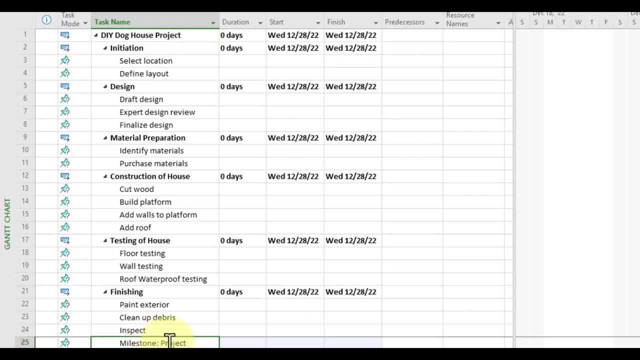 You'll notice that this milestone is indented underneath the group for finishing, So let's outdent it by selecting the task and pressing alt plus shift plus left arrow. The next thing we need to do is to make sure that all tasks are linked correctly to each other. 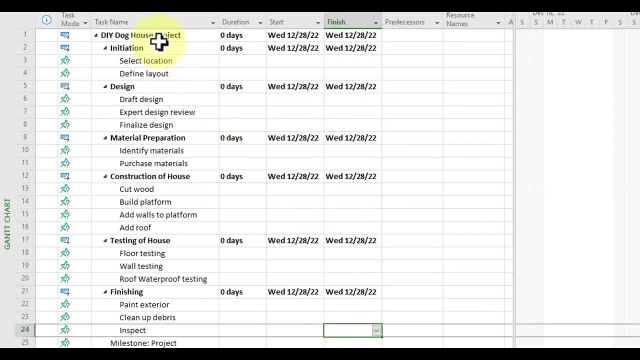 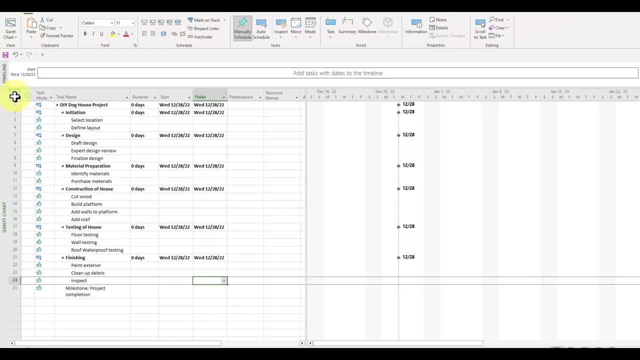 So let's first make sure that Microsoft Project automatically schedules all tasks based upon their dependencies, the resources and the working days in the calendar. To select all the tasks, move your mouse to the top left square button of your table and left click it. 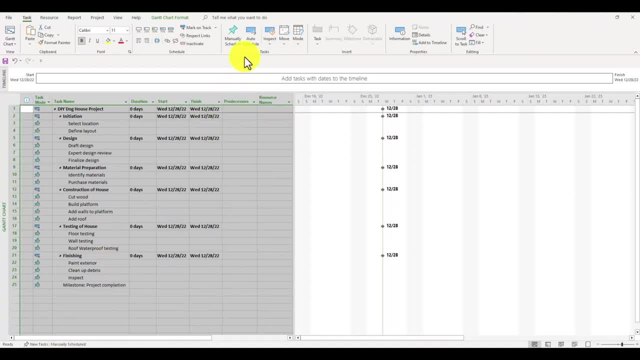 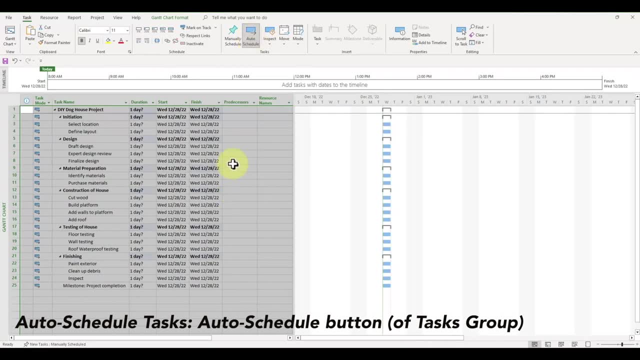 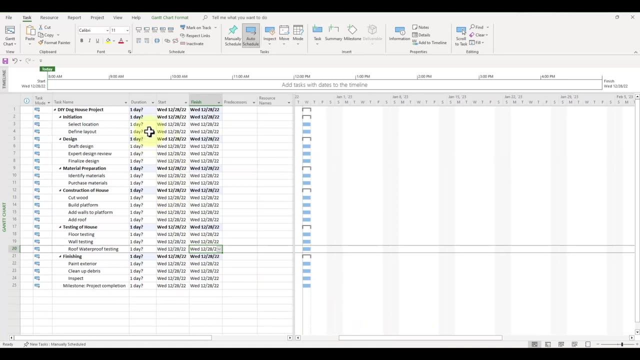 You'll see that all of your tasks have been selected. Now move your mouse to the auto schedule button that's underneath the table. Once you select it, Microsoft Project will automatically input temporary dates and durations, which we'll fix later. The next step to create our schedule is to establish the sequencing of activities. 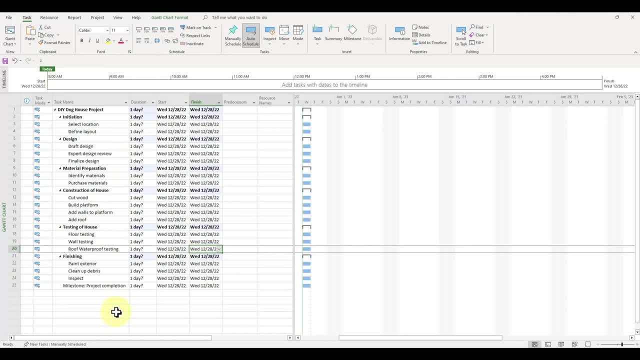 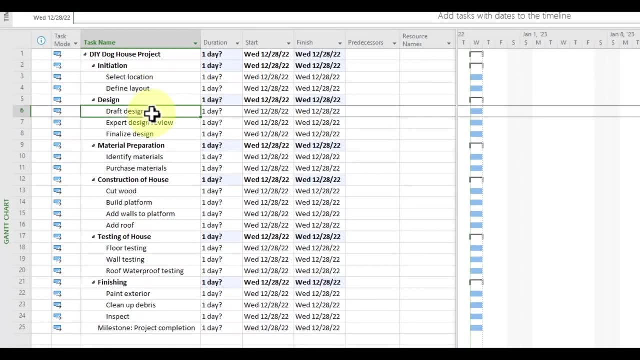 As best practice, we want to add predecessors for the sub-level tasks and not the header group titles. So, starting with the first phase of initiation, selecting the location and defining the layout would happen first at the same time, so both of these tasks would not have any predecessors For the second phase of design, drafting the 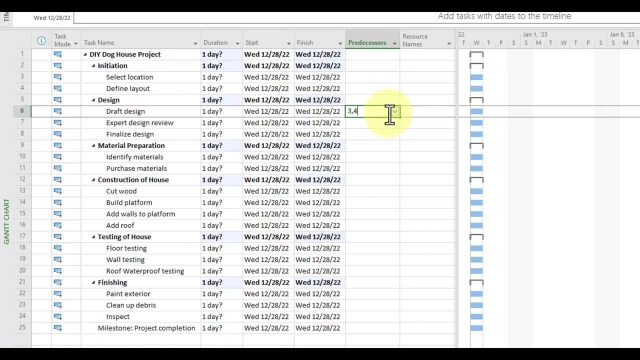 design can only take place after the layout and the location has been identified. We select the location and the layout of the house first, and then we start drafting the design. So for this task, underneath the predecessors column, let's add task IDs three and four. 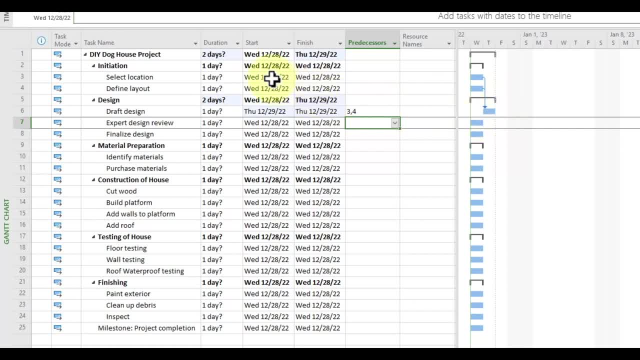 You'll see that the Gantt chart on the right hand side has been updated with this dependency. The first two tasks have been linked to the third task for drafting the design with an arrow. What this tells us is that the first two tasks must take place before the third task can start Establishing. 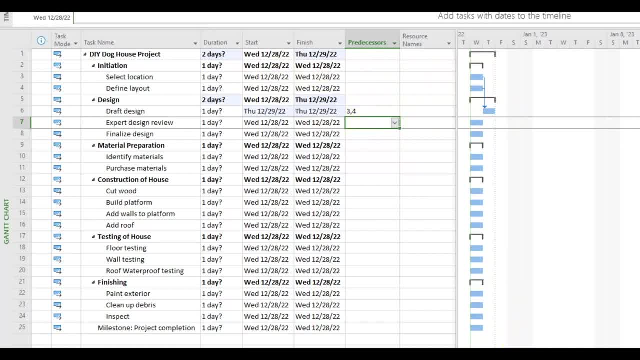 these dependencies is very important so that Microsoft Project knows in what order to schedule each task. Now let's go through the rest of the tasks. So expert design review can only take place after the design has been drafted. So let's add task ID six as a predecessor to expert. 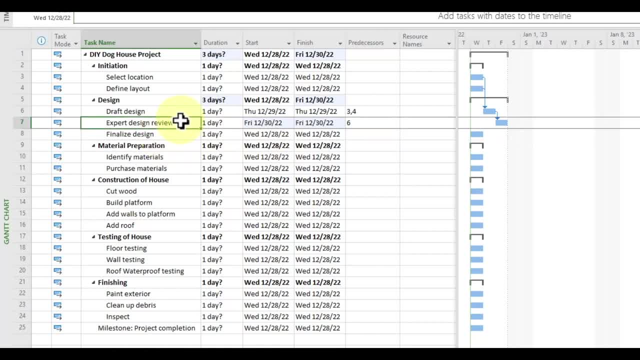 design review. The next task for finalizing the design can only start after you've completed a design review. So let's add task ID seven as a predecessor to finalizing the design, And, just like before, the Gantt chart on the right hand side has been updated automatically. 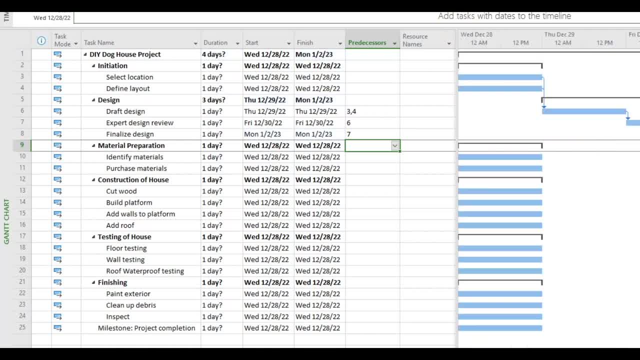 to show these new dependencies, These new tasks must happen sequentially, one after the other, after the design has been drafted. Now let's take a look at the next section. for material preparation, Identifying materials can happen at the same time that you're drafting the design. 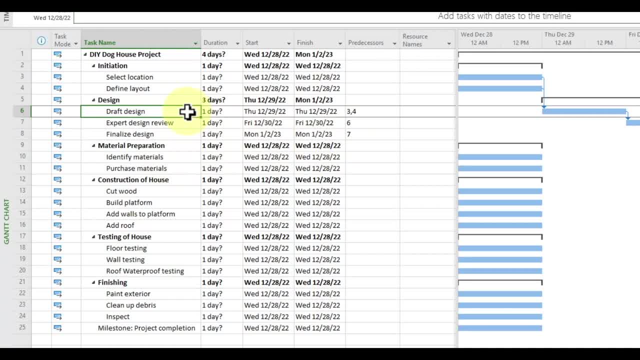 So we want identifying materials to have the same predecessors as a task for draft design. So let's copy the predecessors for task ID six by selecting the cell and pressing control plus C, and then pasting them for task ID 10 by pressing control plus V. The Gantt chart. 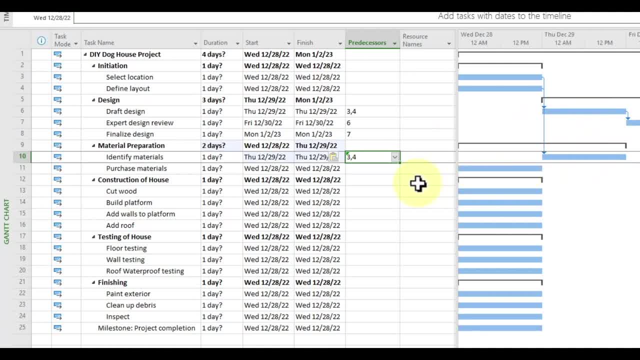 now shows these two tasks taking place simultaneously with the same predecessors. As best practice and as a pro tip, I recommend looking at your Gantt chart to make sure the correct dependencies are in place between each task. The next task for purchasing material can only begin after we've identified the materials, So let's add task ID 10- identify- 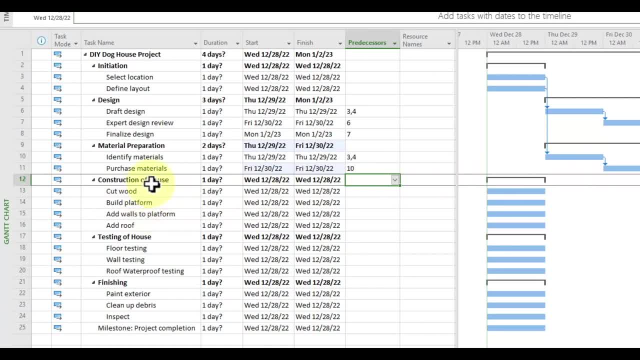 materials as a predecessor to purchasing the materials Moving on to the next phase for construction of the house, we will first cut the wood. We can only cut the wood after we've purchased all of the materials, So its predecessor will be task ID 11.. The next: 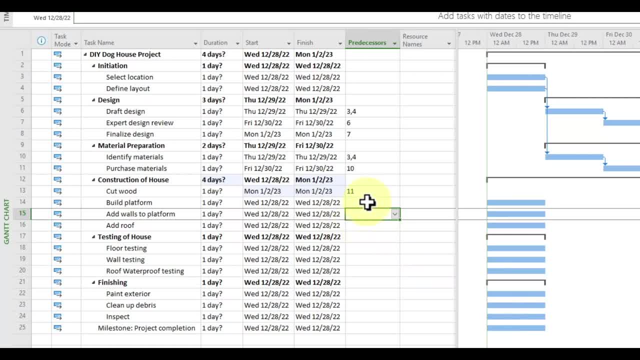 task for building the platform can only start after the design has been finalized, all material has been purchased and the wood has been cut. So this task will have three predecessors: task ID eight for finalizing the design. task ID 11 for purchasing the materials. 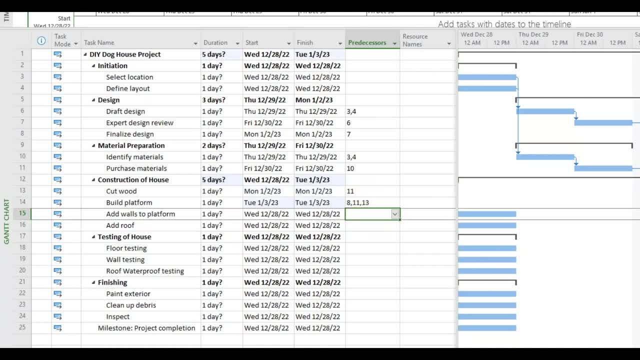 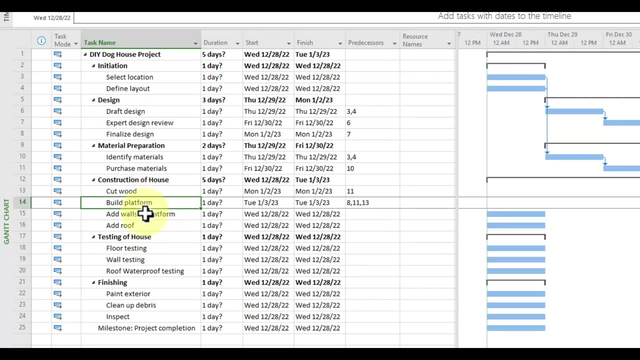 and task ID 13 for cutting the wood. So let's add task IDs eight, 11, and 13, as the predecessors for building the platform. The next two tasks are adding walls to the platform and adding the roof. So, in terms of sequencing the activities, the platform must 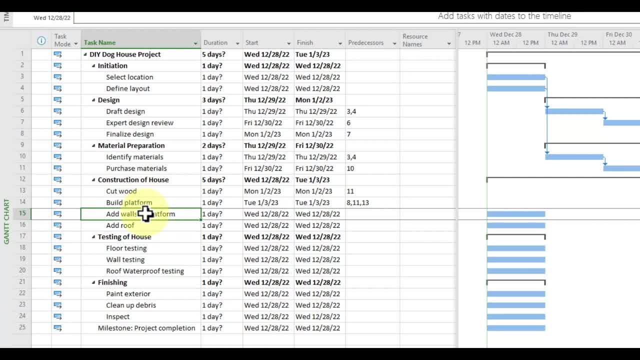 be built first, and then the walls can be added to the platform. Once that's finished, then the roof can be added onto the walls. Since all three of these tasks must happen one after the other, we can use a shortcut in Microsoft Project to quickly link these tasks so they take place in 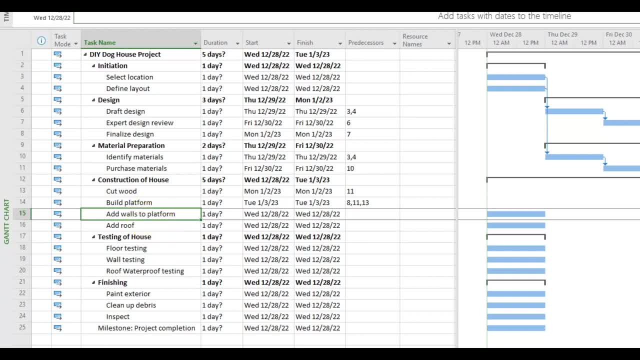 sequential order. We can use the shortcut in Microsoft Project to quickly link these tasks so they take place in sequential order. We can use the shortcut in Microsoft Project to quickly link these tasks so they take place in sequential order. To do that we'll use the chain button of the schedule group underneath the task tab First. 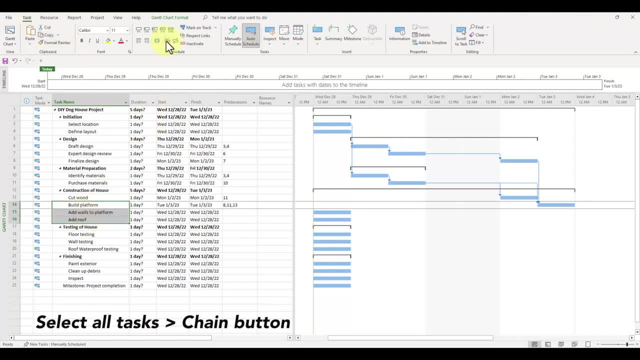 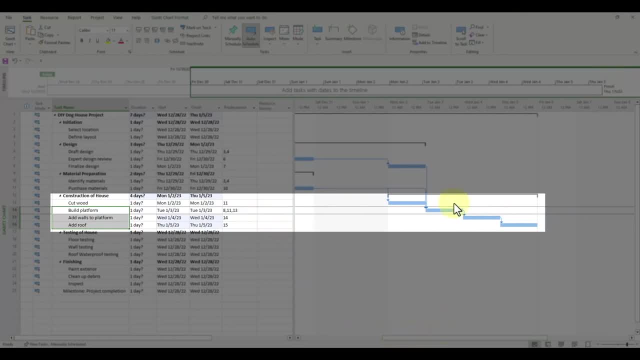 select all three task IDs- 14,, 15, and 16, and then press the chain button. The Gantt chart now shows that all three tasks happen one after the other. One task can't start until the other task has finished in a linear sequence. All right, so going to our next phase for testing of the house. 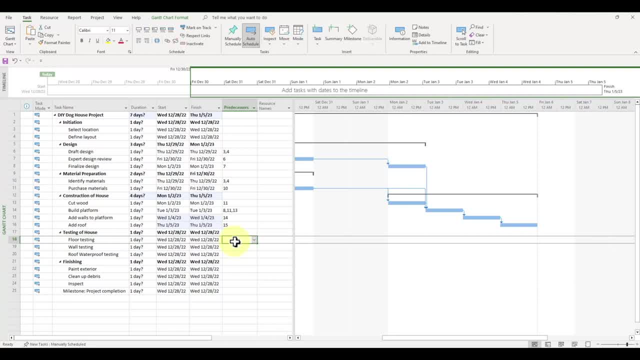 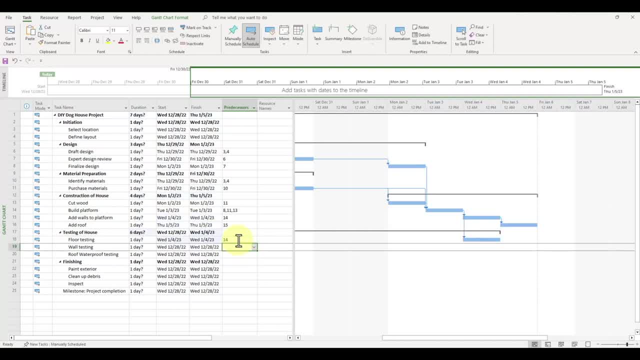 platform has been built, So let's add task ID 14 as our predecessor to floor testing. Wall testing can only start after the walls have been added to the platform, So let's add task ID 15 as its predecessor, And similarly, waterproof testing of the roof. 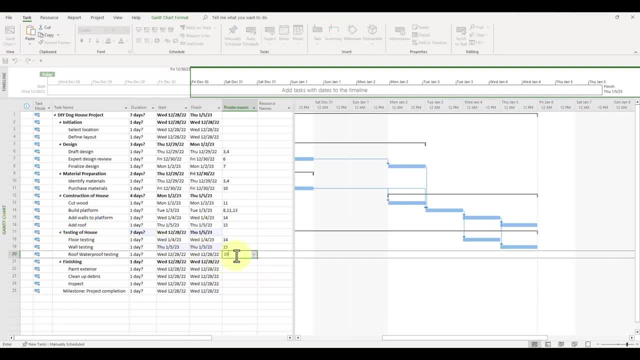 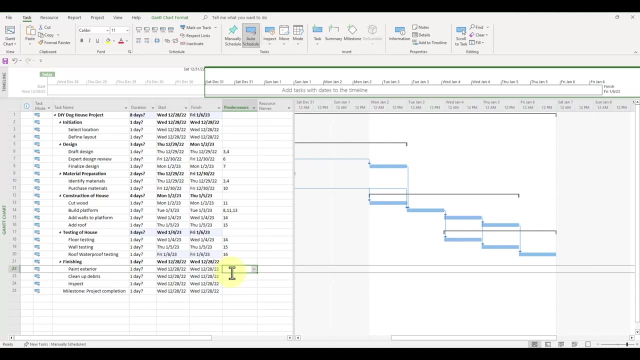 can only start after the roof has been added. Moving on to our next phase for finishing, we have painting the exterior of the house. Let's say that we only want this to start after all testing has been completed and after the roof has been added, So we'll need to add all four of these. 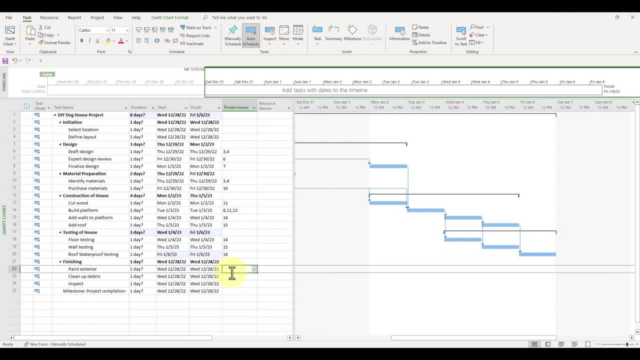 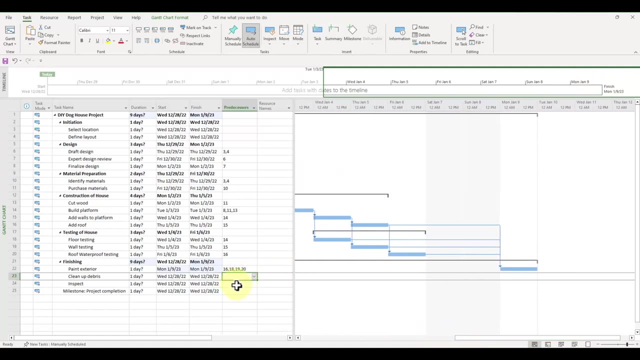 tasks as the predecessors to painting the exterior. All right, so we've added in task ID 16,, 18,, 19, and 20 as predecessors to the task for painting the exterior. The next two tasks for cleaning up the debris and inspecting the house must happen sequentially. 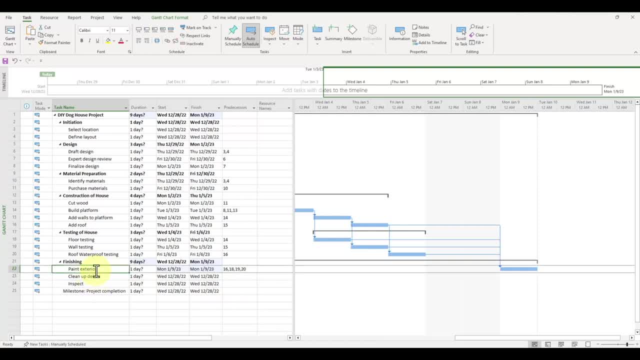 after the exterior has been painted. So let's use the chain button to link these tasks as predecessors, in sequential order, And let's say that the milestone for completing the project will happen after the inspection of the house is completed. So let's add that task as our 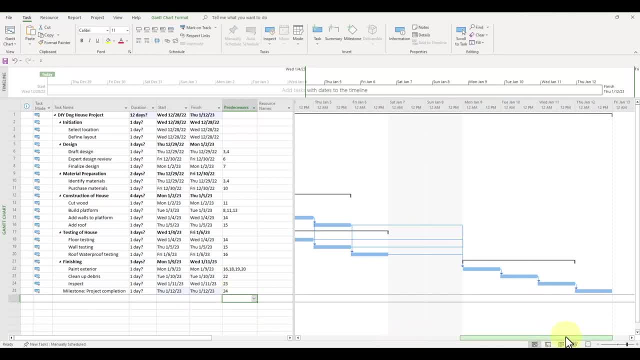 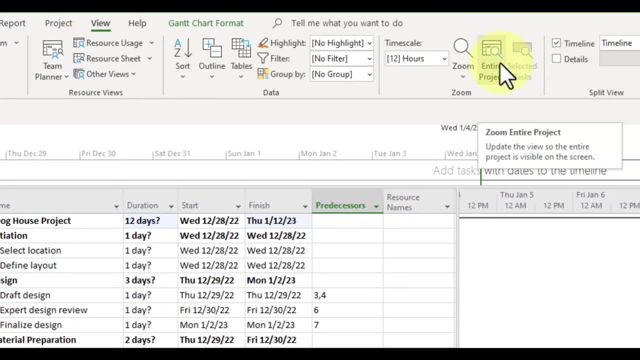 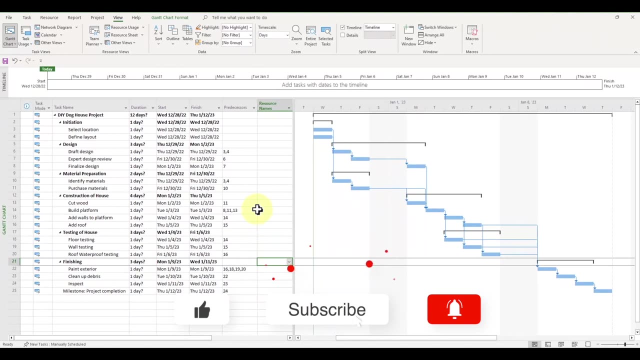 predecessor. Now we can quickly see the overall project view in the Gantt chart by going to the view tab and selecting the entire project from the zoom group. By the way, if you're getting a lot of value out of this video, do me a favor and smash that like button. It truly shows your support for. 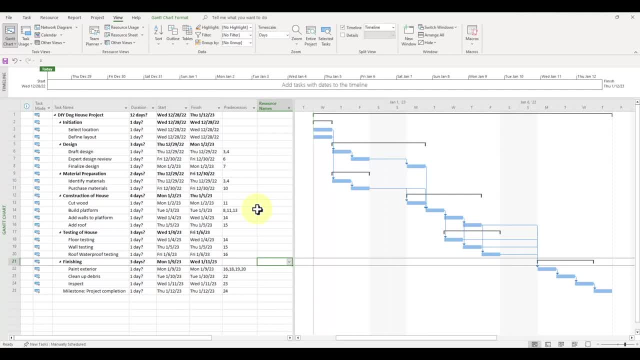 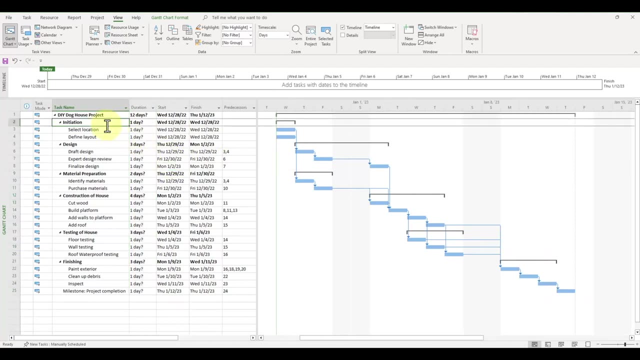 me and it helps the channel tremendously so I can make even better videos like this. All right, now that we added in the correct dependencies for all tasks, the next step is to determine the durations and how long each task will take. For the initiation phase, let's say: 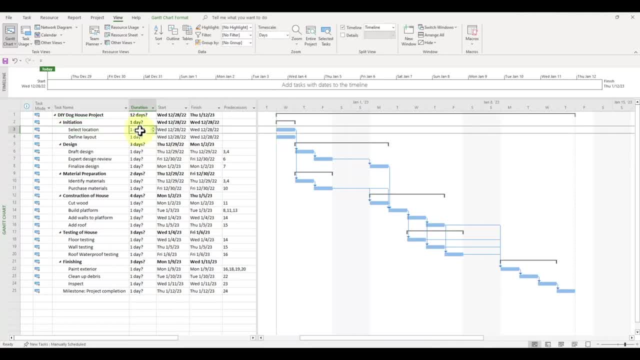 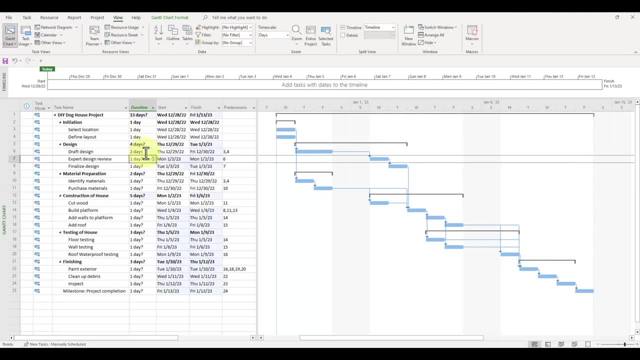 that selecting the location and defining the layout will take one day each For the design phase. let's say that drafting the design takes two days, while the design review and finalizing the design only take one day each. For the next phase of material preparation, we'll be identifying: 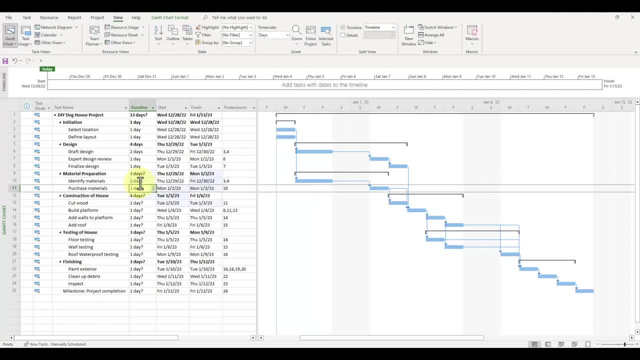 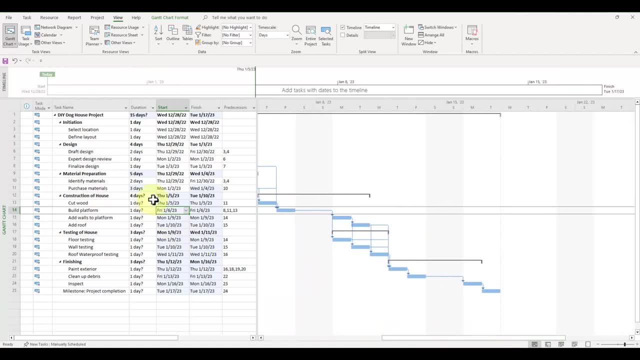 materials, which will take two days, and purchasing materials- let's give it three days. All right, so let's go down to the next phase for construction of the house: Cutting the wood should only take one day. Building the platform, adding the walls. 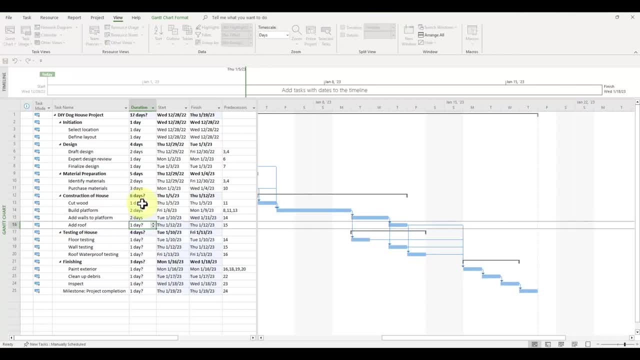 and adding the roof should each take about two days days long For testing of the house: testing the floors, the walls and the roof. that should all take one day each. So for the finishing phase, let's also say that painting the exterior, 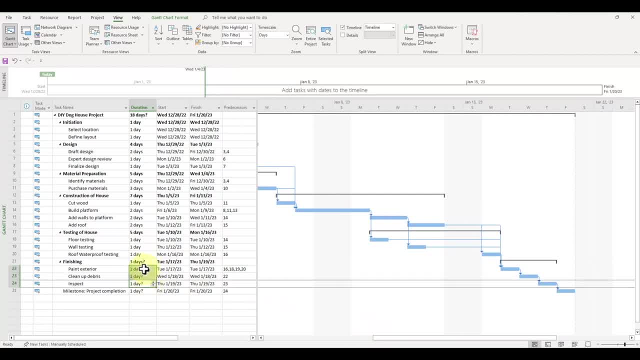 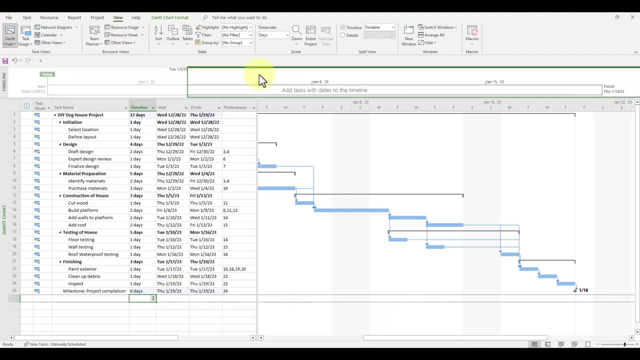 cleaning up all the debris and inspecting the final house also take one day each. And for the milestone signifying the project completion. since this is a milestone, this should not have any duration assigned to it, so let's give it zero days Now when we zoom out of. 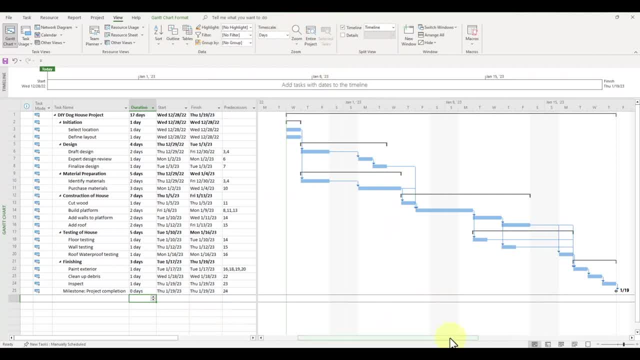 the GAN chart, we can see the entire project timeline with the correct duration. By this point we've established all the tasks in our project. We've also defined the correct predecessors for each task, or in other words, the correct sequencing of activities, And we've also 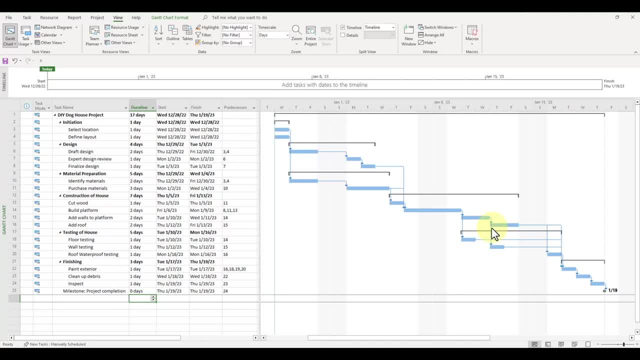 determined the durations for each task or the best case estimates for how long it will take to complete the work. The next step for us is to assign resources to each task. To do that, we need to change our view from GAN chart to resources mode. So move your mouse to the leftmost side of the screen, where 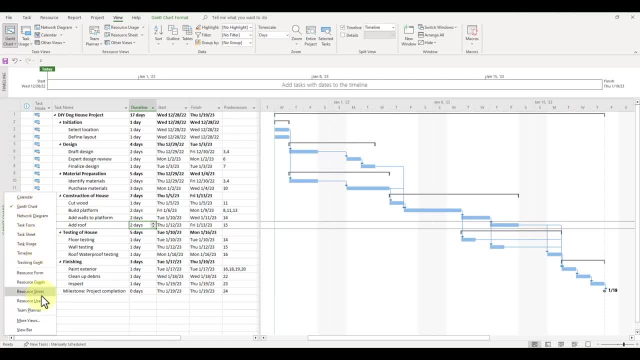 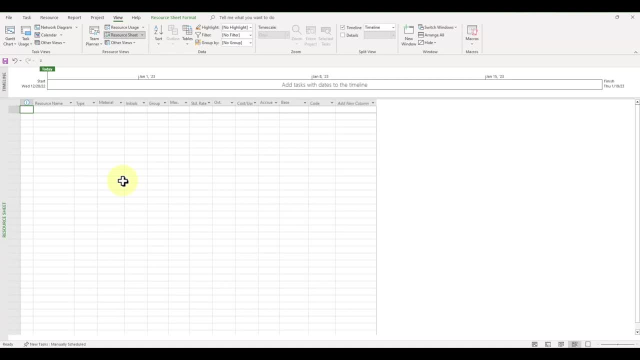 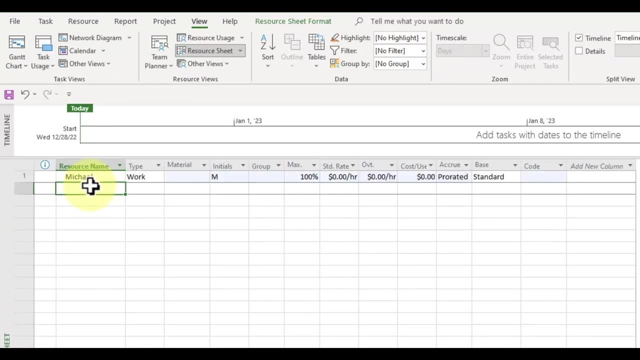 it says GAN chart. Right click and select the option for resource sheet. This is the section within Microsoft Project where we'll list out the material and all the labor resources that we'll use on our project. Let's say that there are three people working on this project: Michael. 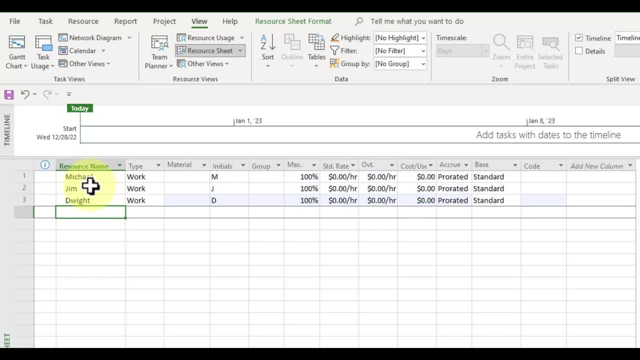 Jim and Dwight For the material that we're using. let's add wooden planks and nails And let's say that we'll be hiring contractor A to cut the wood for us. After we've added these resources, we need to make sure that the material types are correct. Michael, Jim and Dwight are 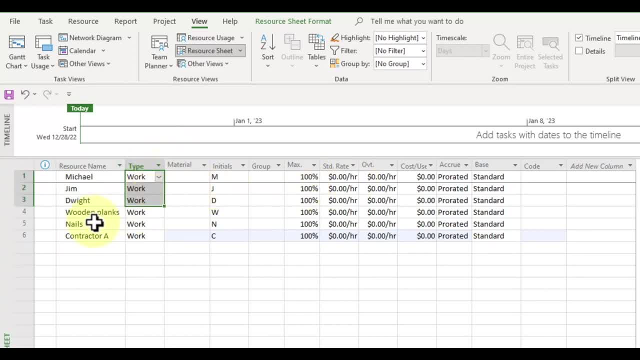 individuals who will work on the project on an hourly rate. so this is correct. The wooden planks and the nails are both material types, so let's select that option from the drop down menu. We'll be working with contractor A to cut the wooden planks for us, so this will be a service. 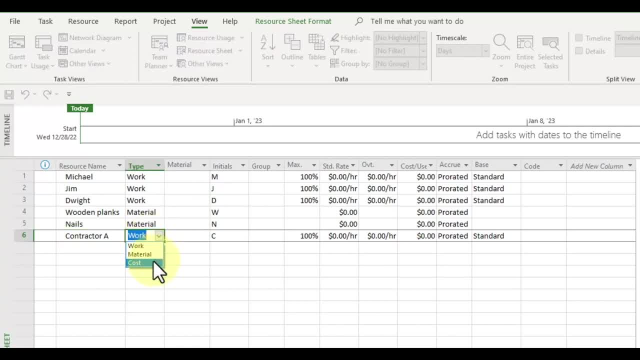 or a cost to the project itself. So let's change this material type from work to cost. Now let's assign the hourly work rates for Michael, Jim and Dwight. For Michael, let's say that he gets paid a standard rate of $30 an hour And both Jim and Dwight are paid $25 an hour For the wooden 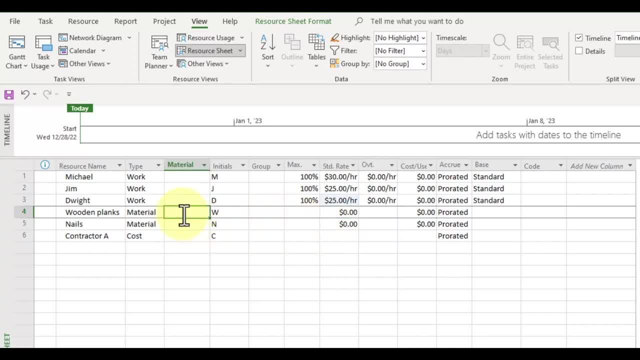 planks, let's say this is priced in terms of linear feet, so three dollars and fifty cents per linear foot. And for the nails, let's say that this is priced at $7 per box and each box contains 100 nails. For our contractor A, let's say that we'll pay them after all their assigned. 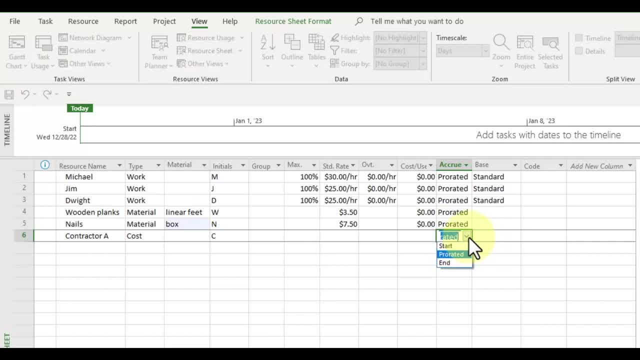 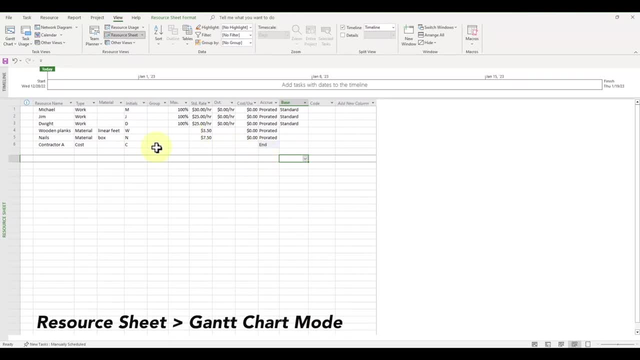 work with cutting the wood is completed. So instead of putting prorated, we want to pay them at the end of that activity. Now that we've defined all the resources, let's switch out our resource sheet mode and go back to the Gantt chart mode, so we can assign our resources to. 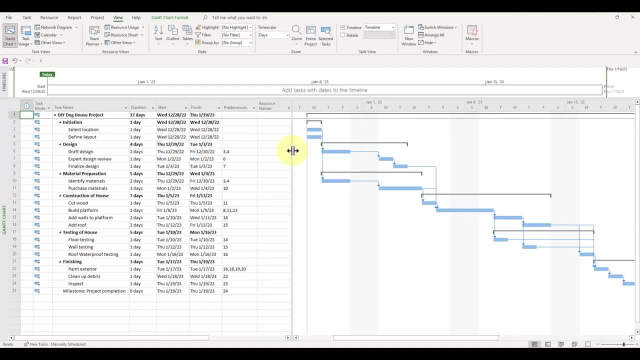 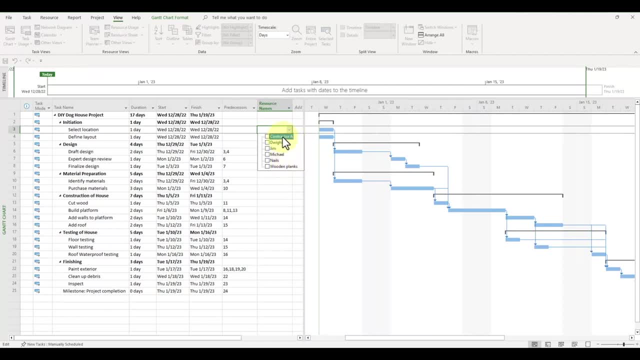 our project's tasks. In the column for resource names, you should see a drop down menu for each resource. However, I found that it can be very tedious and really time consuming to assign resources to every single task using this approach. Instead, if you're assigning resources, 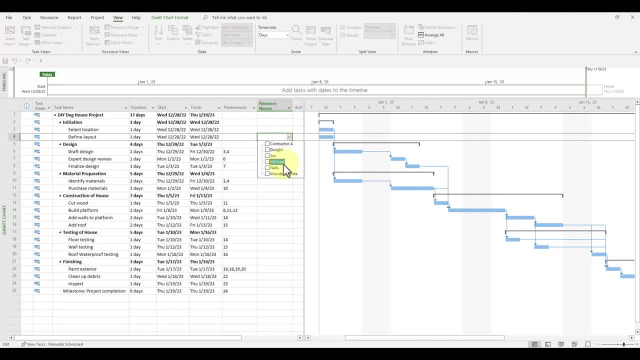 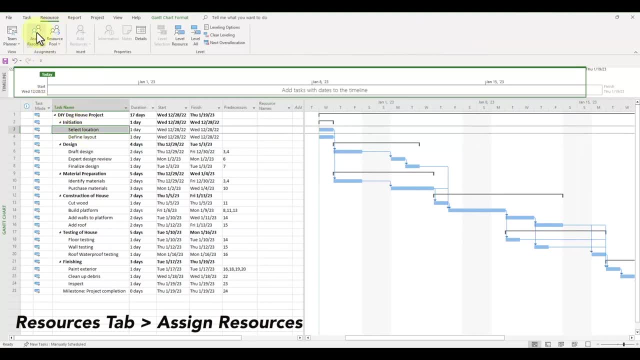 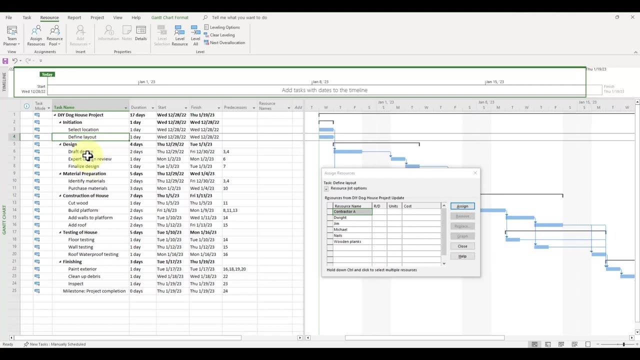 to multiple tasks simultaneously. here's what I personally recommend: Go to the resource tab and click on the button for Assign Resources, Which is a part of the Assignments group. What I love about this feature is that you can assign more than one task to multiple resources all at the same time, And you can see that the task name 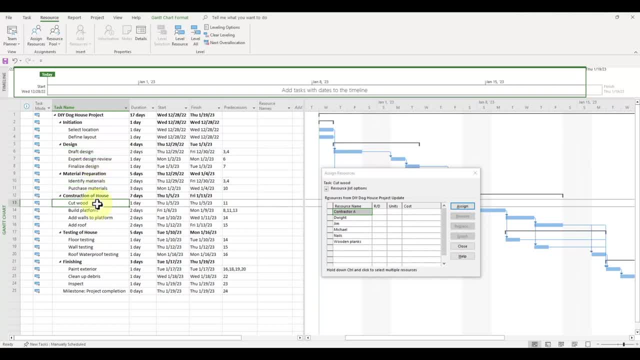 changes inside the window when I select a new task. So let's assign Michael to the tasks Select Location, Define Layout and Inspect. To do that, press the control key and left click each of the tasks In the Assign Resources window. click on Assign Resources. 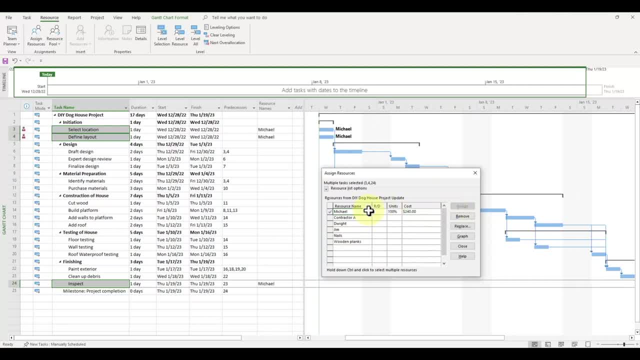 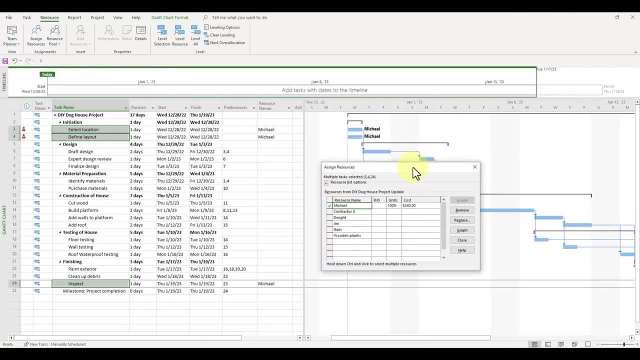 Click on Michael and then click on Assign. Immediately we can see that Michael has been assigned as a resource and the cost for his work is $240.. So now let's assign Dwight to Draft Design Expert Design Review, Finalize Design, Paint Exterior and Clean Up Debris. 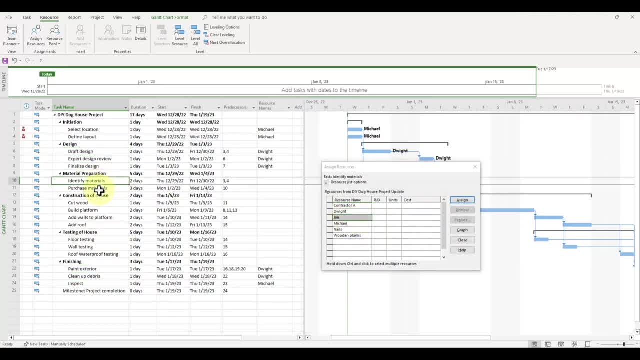 For Jim, let's assign him to all the tasks for Material Preparation, Construction of the House, Except for Cutting the Wood and, of course, Testing the House. And let's assign Contractor A to Cut the Wood for a one-time service cost of $20.. 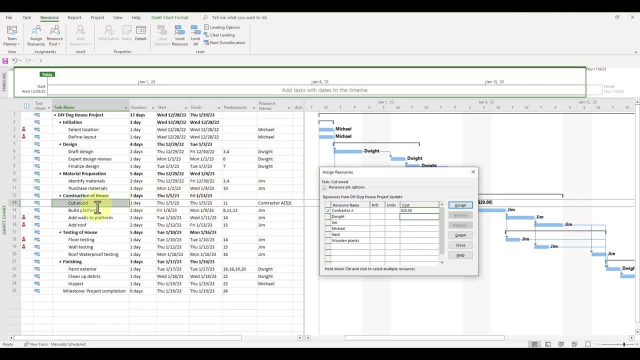 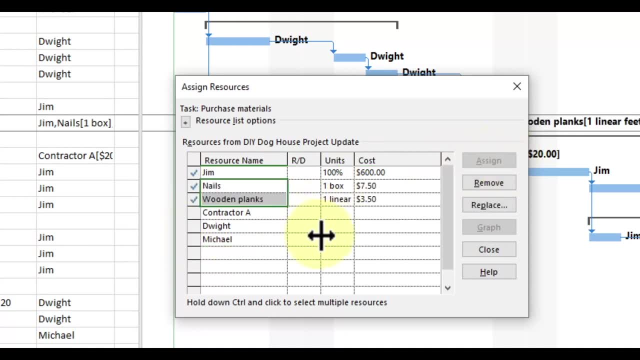 All that's left to do is to assign our material resources. So let's assign Nails and Wooden Planks to the task for Purchase Materials. Right now, Microsoft Project is saying that we only need one box of nails and one linear foot of wooden planks. Let's say that we actually need. 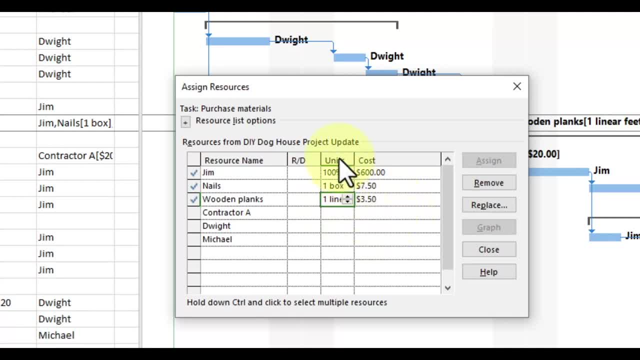 10 linear feet of wooden planks. So to do that underneath the Units column. change the name of the task to Nails and Wooden Planks. To do that underneath the Units column. change the name of the task to Nails and Wooden Planks. To do that underneath the Units column. 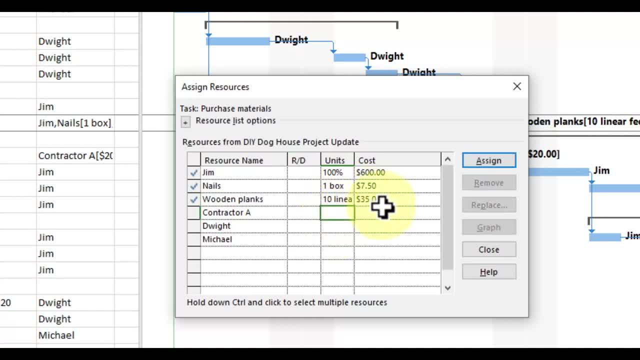 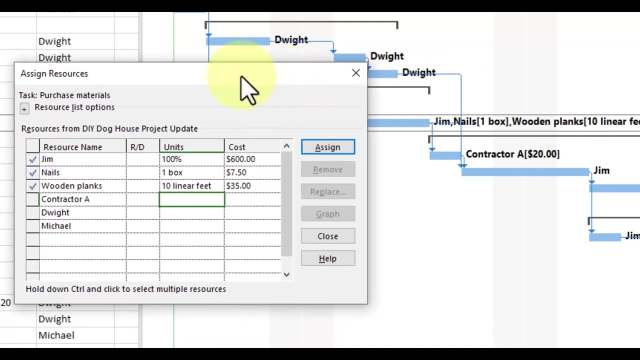 change it from 1 to 10.. Right away we see that the cost of all the wooden planks has changed from $3.50 to a total of $35.. Now when Microsoft Project calculates the cost for our project, it's going to assume that we're purchasing 10 linear feet of wooden planks and $35 for a cost. 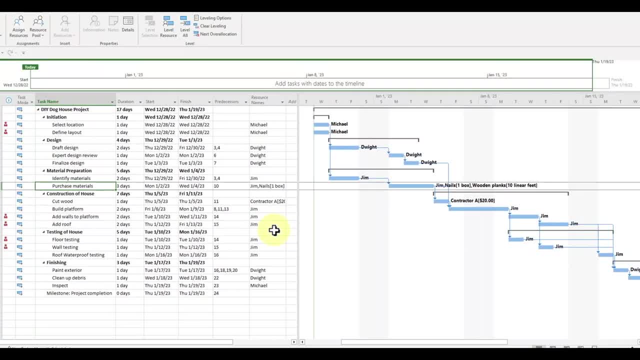 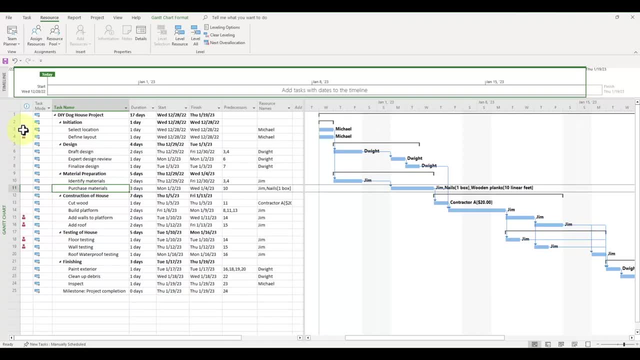 estimate. We've now assigned all resources to our tasks. But if you look to the leftmost column for Indicators, we see a red person icon which tells us that we've assigned all resources to our tasks, Which tells us that a resource is over-allocated for these tasks. To better visualize where our 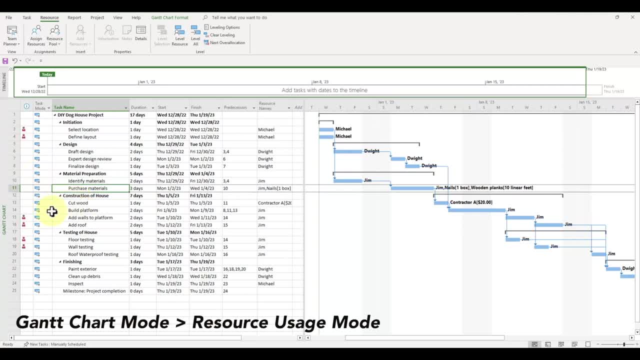 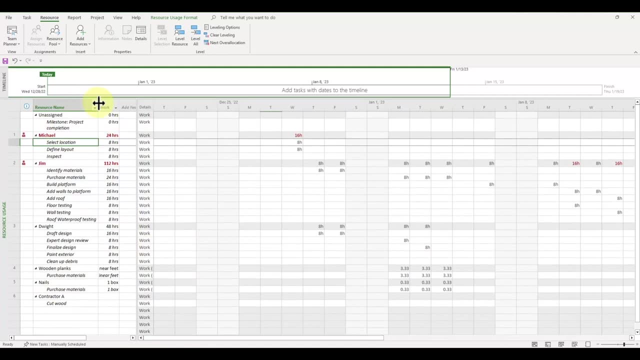 resource over-allocation is. let's switch from Gantt chart mode to resource usage mode. To do that, go to the left side of your screen where it says Gantt chart, right-click and select Resource Usage. Inside Resource Usage mode we can see what task is assigned to a specific resource. 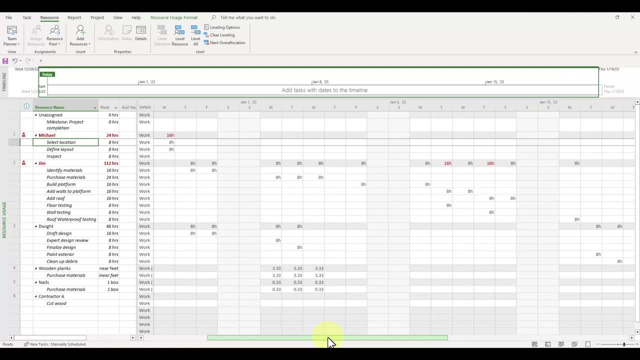 and what date this is taking place on the chart to the right For our project. Michael is over-allocated on two tasks for Select Location and Define Layout. because these two tasks are taking place on the same day, Jim is over-allocated for the. 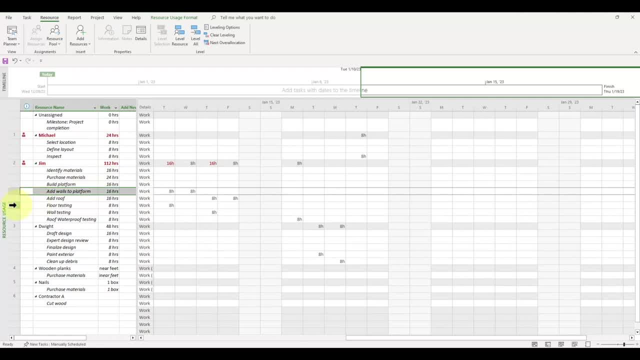 following tasks: Add Walls to Platform and Floor Testing and Add Roof and Wall Testing. To prevent this resource over-allocation, instead of having Jim work on floor testing and wall testing, let's assign Dwight to these two tasks, since he's available for the rest of these dates. So let's switch from Resource Usage to Gantt chart mode. Let's 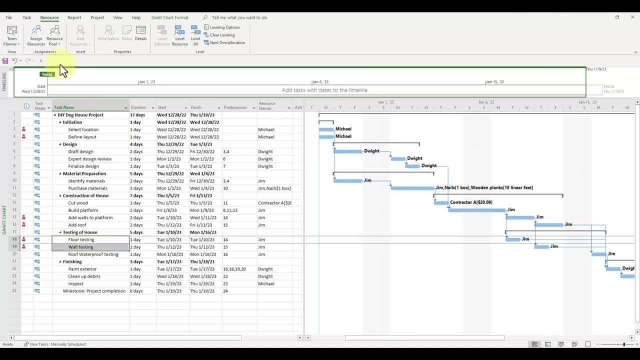 select the two tasks for Floor Testing and Wall Testing and click on Assign Resources. Select Jim and click Remove and then assign Dwight. Alright, so the last resource over-allocation is with Michael for selecting the location and defining the layout. To fix this, let's have Define Layout. 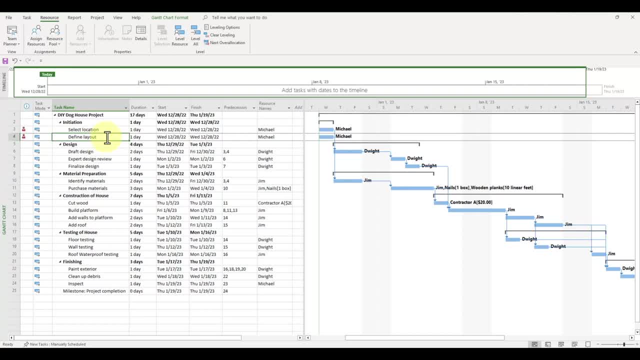 take place after Select Location is finished. So let's add task 3, as a predecessor to defining the layout, With all of our tasks and our resources assigned. let's take a look at the cost for our project. To do that, let's switch our table view, Go to: